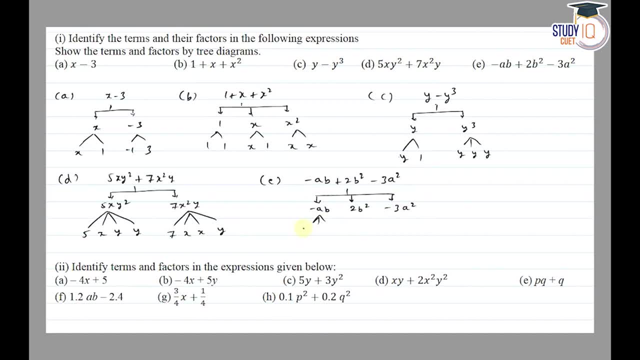 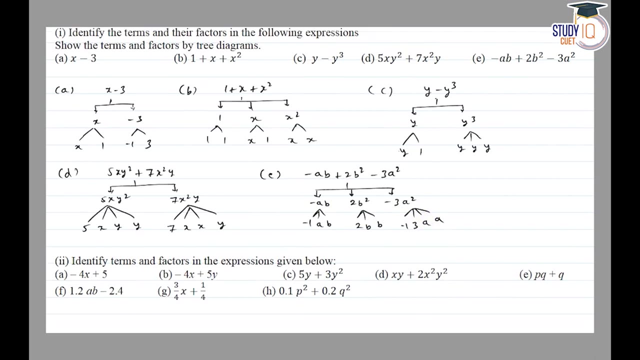 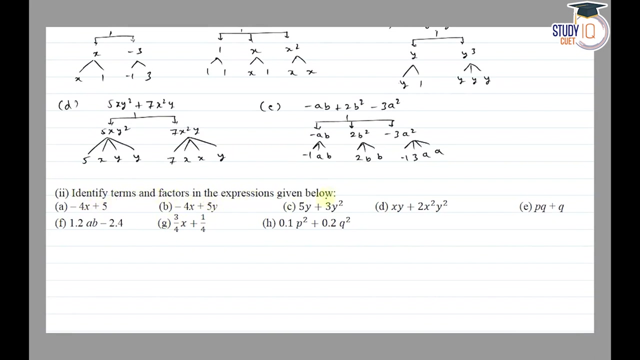 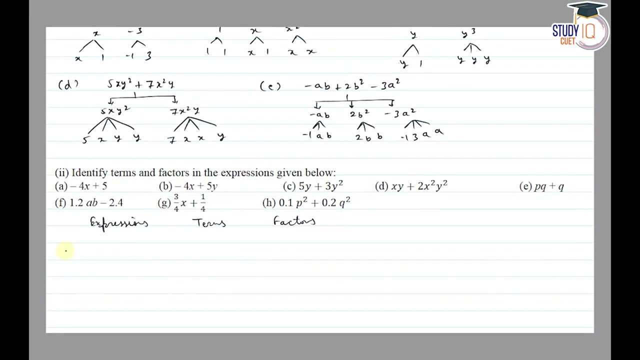 We will have vectors here: Minus 1ab, 2bb and minus 1- 3a. a second part is identify terms and factors in the expression given below. so my expression, given him, i'm a term and factors. find out: minus 4x plus 5. term will be minus 4x and 5. 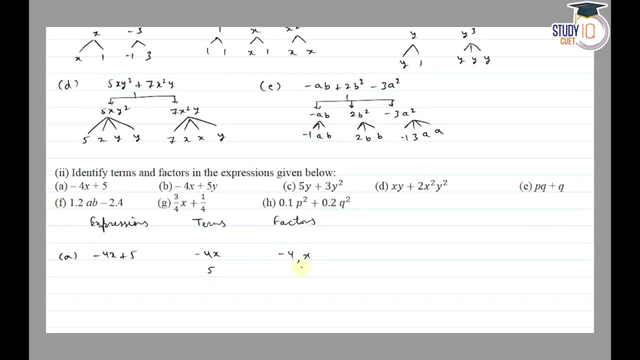 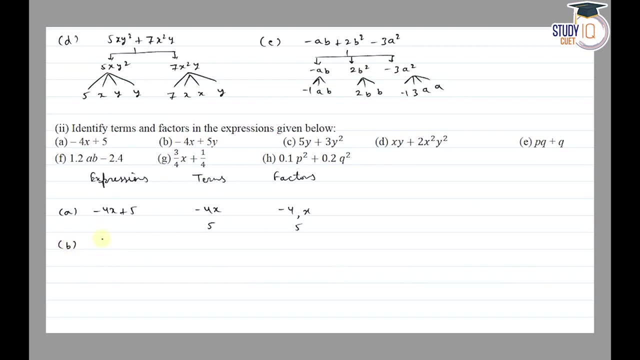 so factors will be minus 4 comma x and 5 b is minus 4x plus 5y. minus 4x and 5y is terms minus 4 comma x and 5 comma y. for part c: 5y plus 3 y square two terms: 5y and 3 y square 5 y and 3 y y. 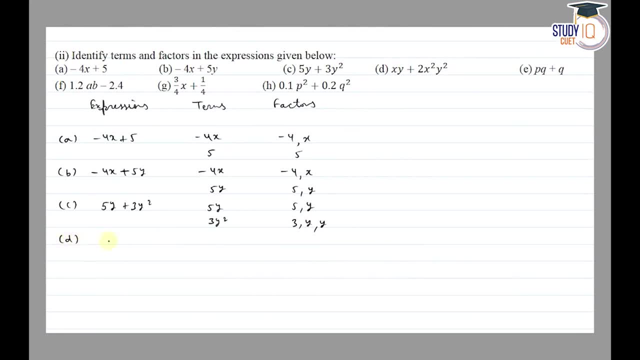 plus. part d is x, y plus 2 x square y square. two terms: x, y and 2 x square y square. factors x, comma y and 2 x comma, x comma, y, comma y. part e is p, q plus q, p, q and q. here two terms: factors b comma, q and q. part f is 1.2 a b minus 2.4. 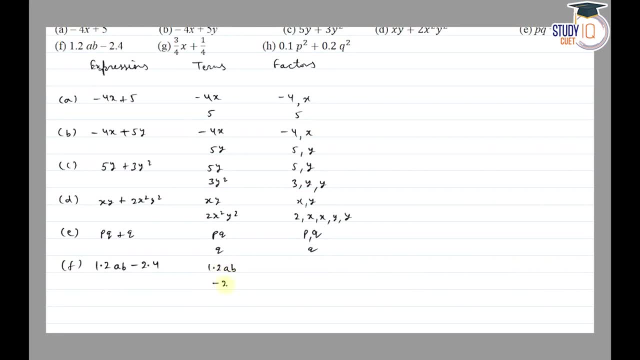 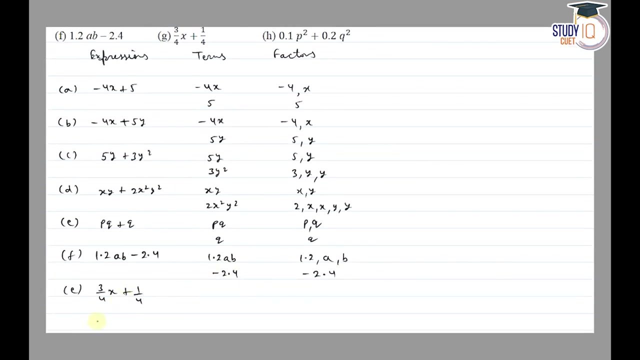 1.2 a, b and minus 2.4. here two terms, one point, two factors: 1.2 comma A, comma B and minus 2.4. part E is 3 by 4x plus 1 by 4 and part H is 0.1 B. 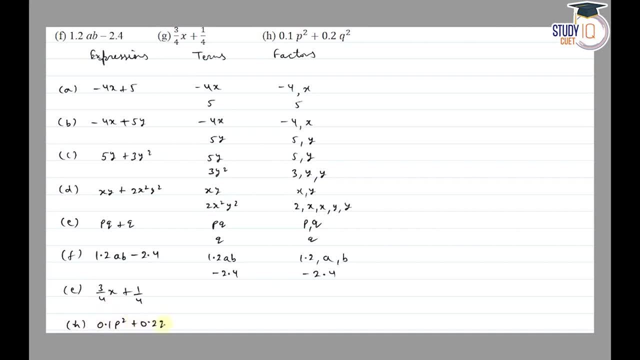 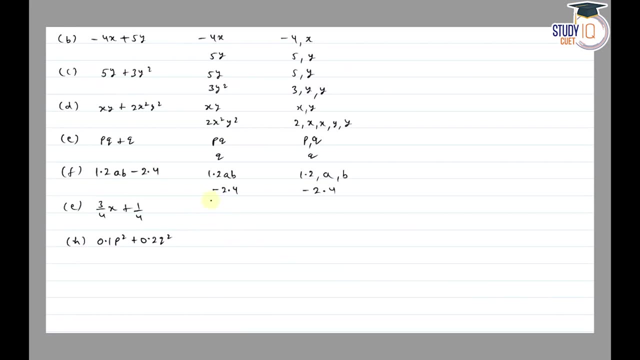 square plus 0.2 Q square. So here terms, two terms, is 3 by 4x and 1 by 4, and factor is 3 by 4 comma x and 1 by 4.. In part H, here two terms: 0.1 B square and 0.2 Q square. factors are: 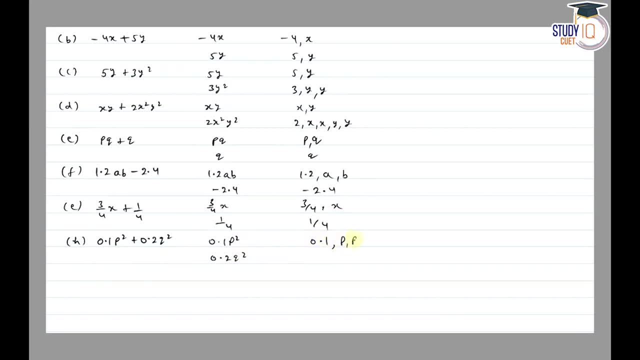 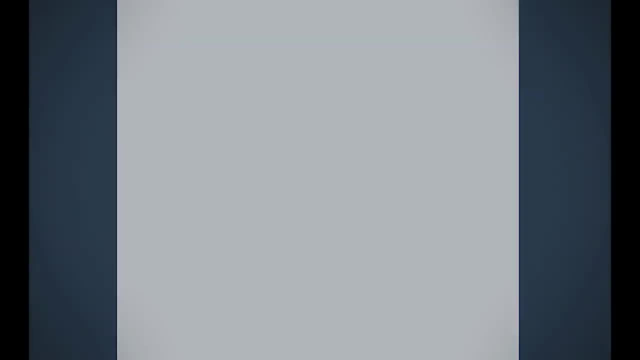 0.1 comma P comma P and 0.2 comma Q comma Q. Thank you. All right, you guys, we're gonna have a busy two weeks because we are going to take this project from start to finish. This is an 11 foot tall retaining wall on a steep slope. We're gonna wrap this job up this week and then next week we're gonna dive into a patio that we're putting on. 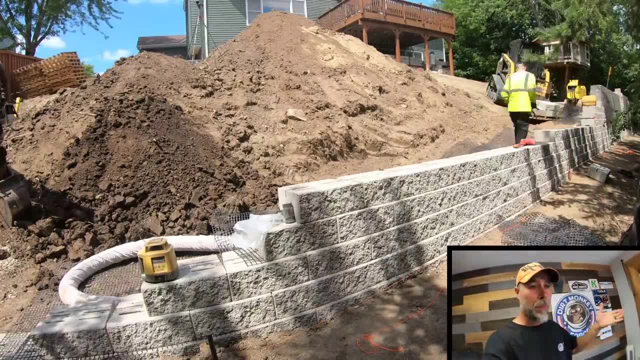 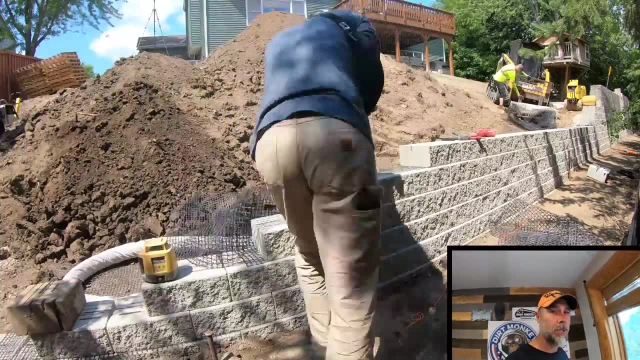 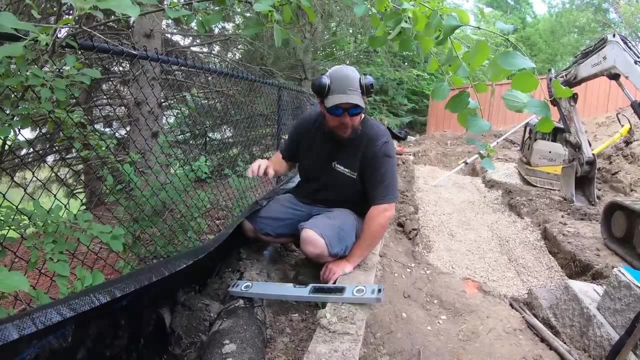 top of this retaining wall and we're gonna show you that series back to back to back so you'll be able to watch this job go from where it's at to final completion without interruption. I guess the grade's changing a little bit here. It's kind of starting to come downhill this way. 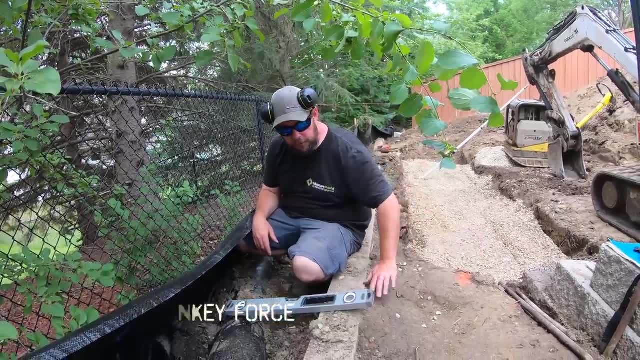 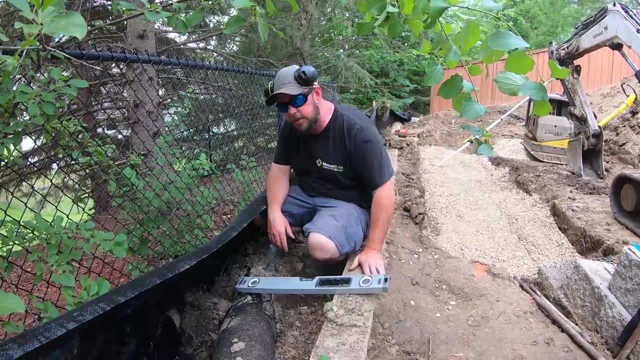 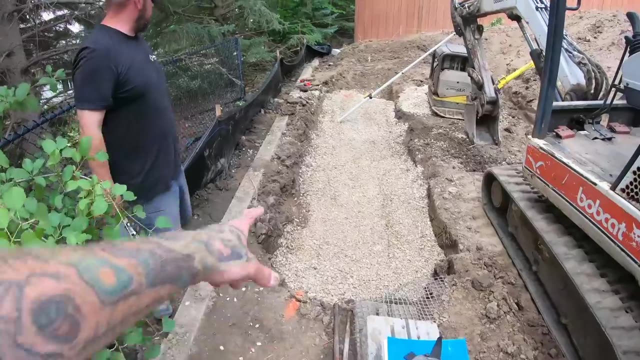 and then this wall is too close. We're shooting for a three to one in front of the wall, We're burying the second block and I don't want to trust anything that this is doing, So we're gonna cut this out of here. It worked over there, but it's not working over here for me. Essentially, we're